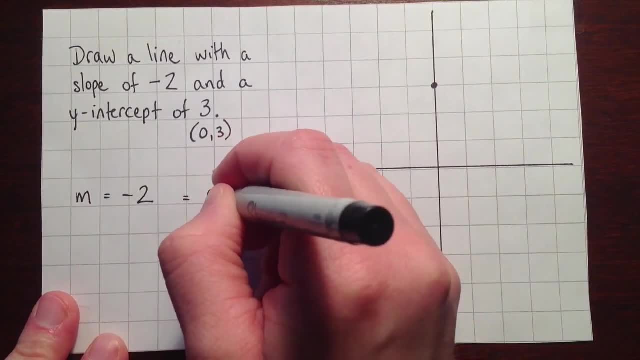 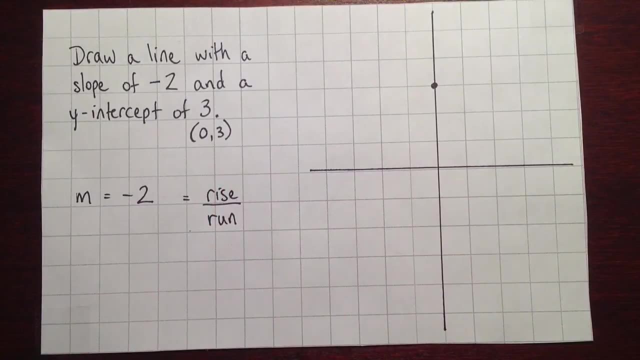 And remember, our slope is rise over run, So if your slope isn't a fraction, the first thing you can always do is just make it into one by calling it: instead of negative 2, it'll be negative 2 over 1.. 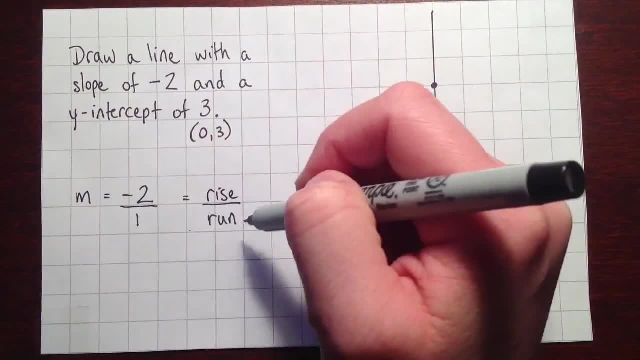 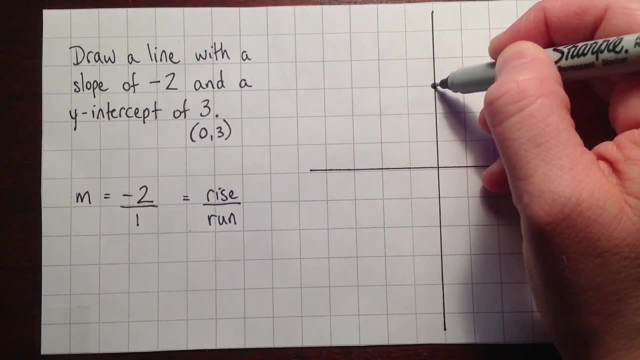 So that means we want to rise negative 2 and then do a run of 1 every time. So we'll start at the point that we know And we'll rise negative 2, so that means we'll go down 2.. And then we'll do a run of 1, so that means we'll go to the right 1.. 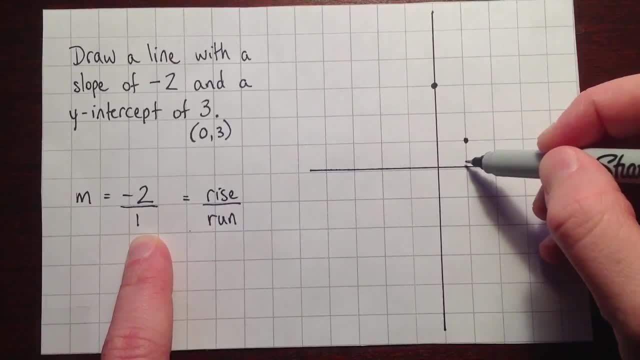 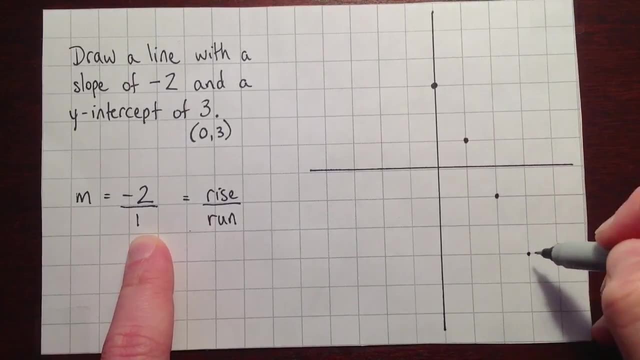 So we'll go through that point And we can do it again: A rise of negative 2 and a run of 1. And we go through that point. It's kind of nice to do it until you get to the edge of your graph. 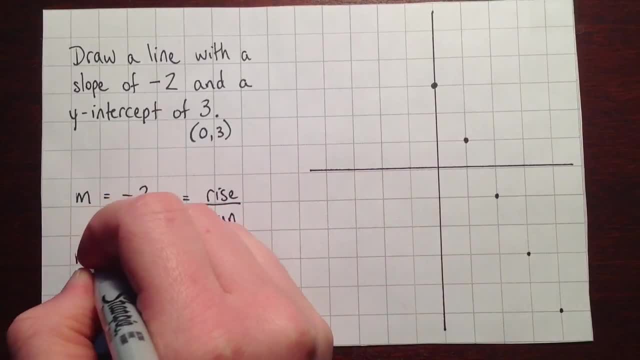 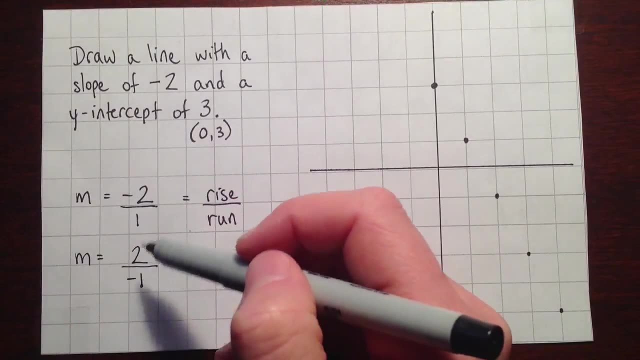 Now, an interesting thing to note is that we could also write negative 2, as we can write it as 2 over negative 1.. Because we can have the negative side of the fraction all the time. So we can write it as the top or the bottom, and it doesn't matter. 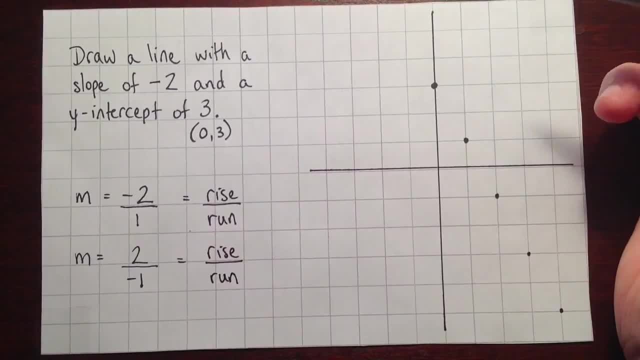 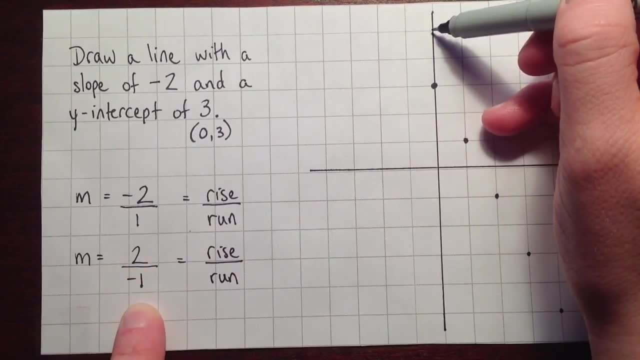 Just whichever you prefer. So in this case, that would mean that we do start at the beginning again. we do a rise of 2, which we go up, 2. And then a run of negative 1, which we go to the left. 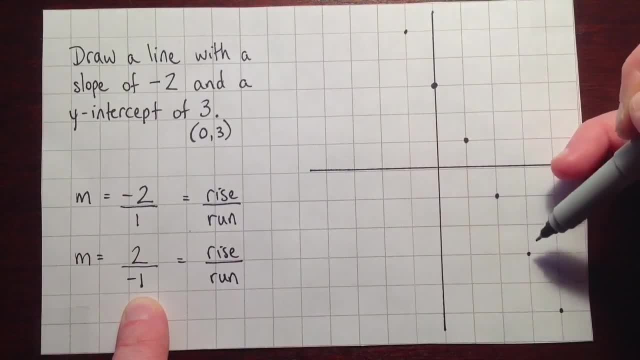 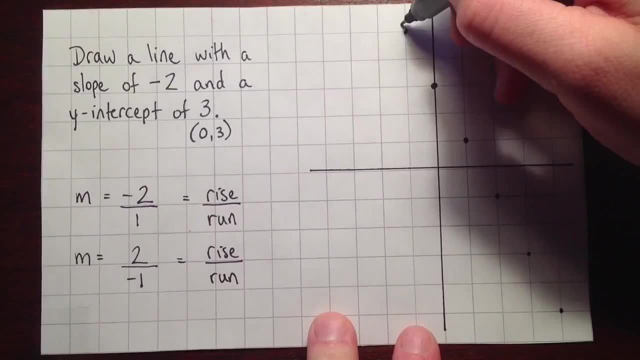 And if we look at that, that makes perfect sense. It's the same thing. It gives us a different point, but those are all in the line there. Okay, Then we'll just Okay. so this is my line through there. 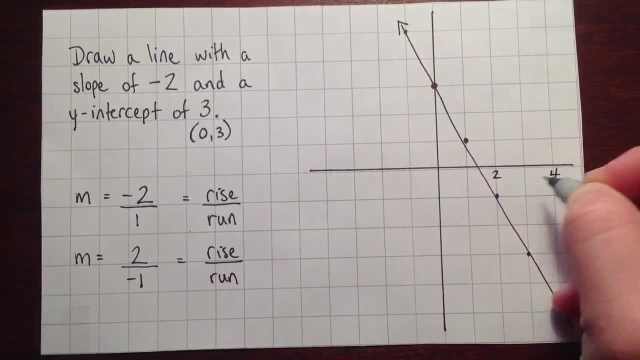 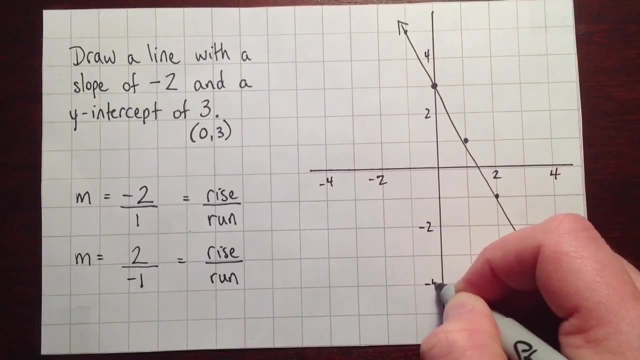 We should probably show here how much we're going up by every time. Okay, So here's the line, with a y-intercept of 3, so that's the point- and a slope of negative 1.. This makes sense because we know that negative slopes go in that direction. 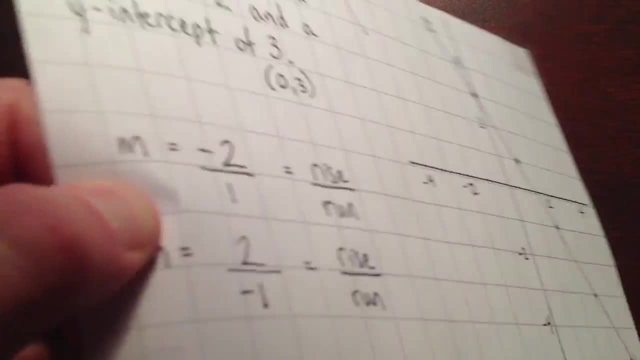 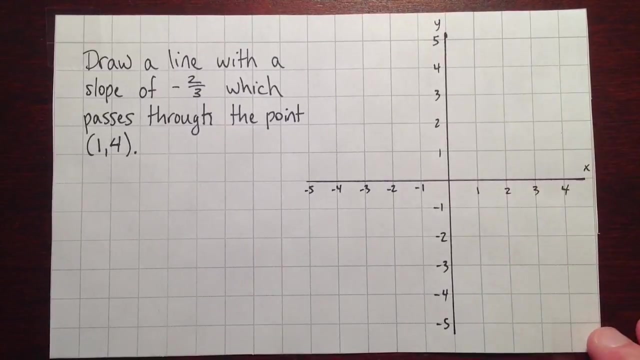 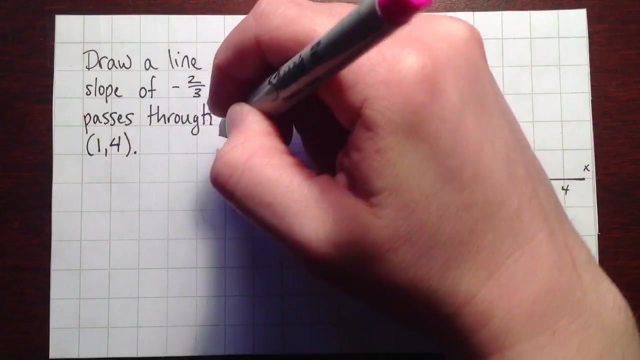 Okay. so for another example, Suppose I wanted to draw a line with a slope of negative 2 thirds that passes through the point. Okay, So before we start we can make a note that again a negative slope would be kind of like this: